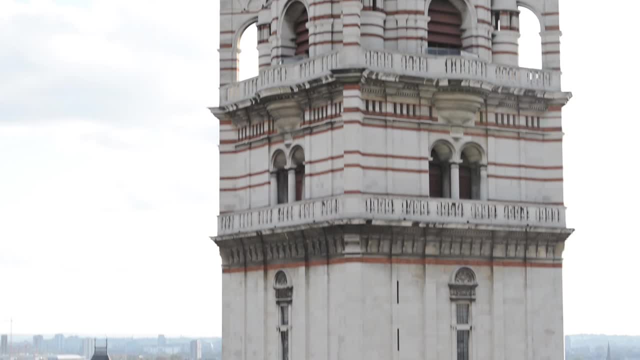 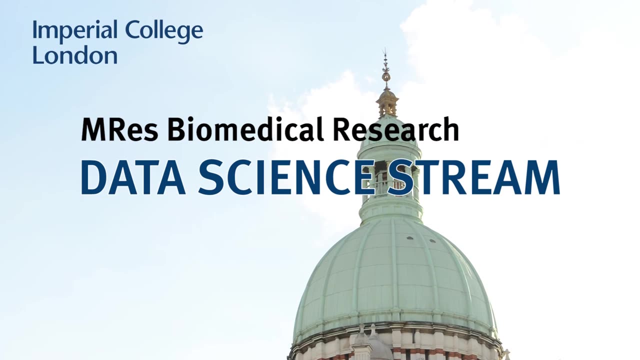 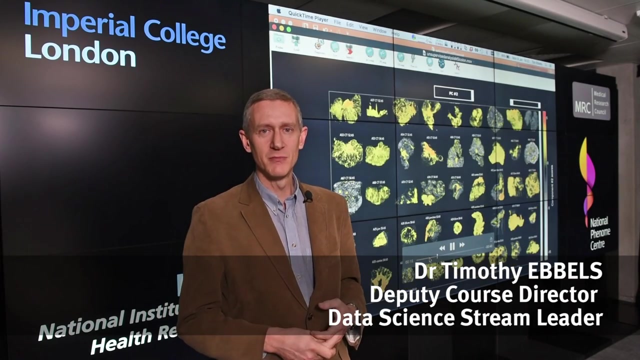 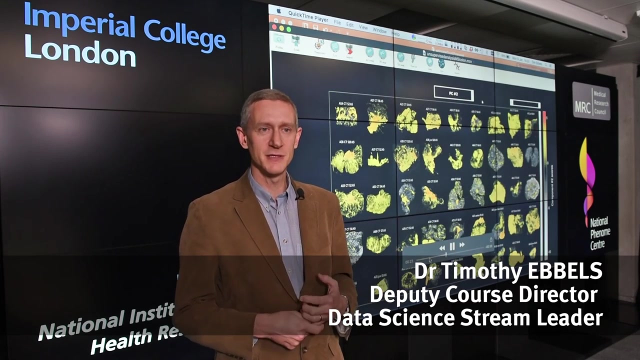 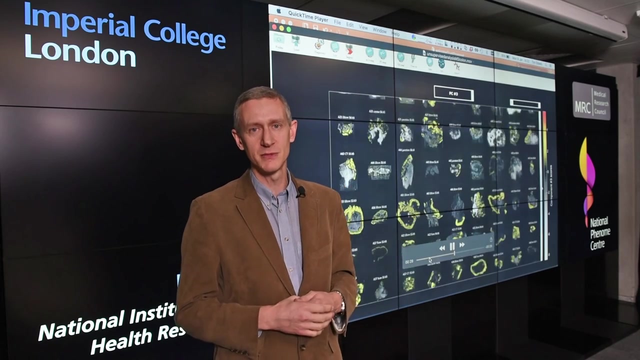 The Data Science Stream on the MRes in Biomedical Research is a course designed for engineers, people with a mathematical and physical sciences background, and it's to give a training in data science applied to biomedical problems. As many of you will know, the world is changing. 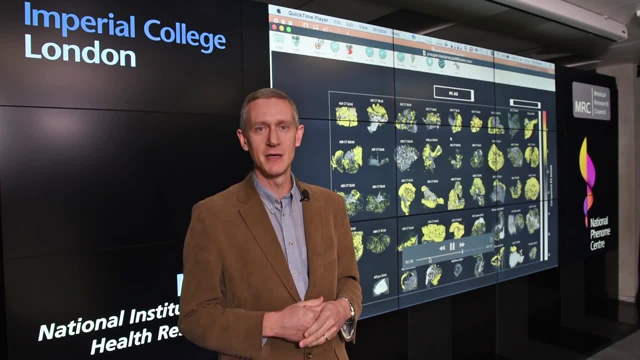 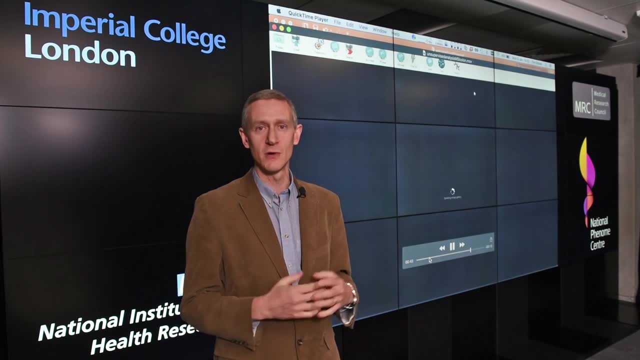 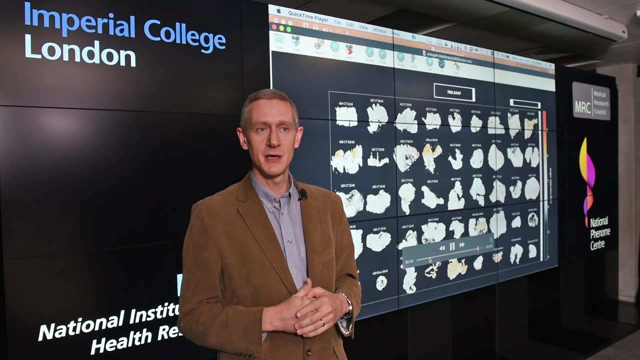 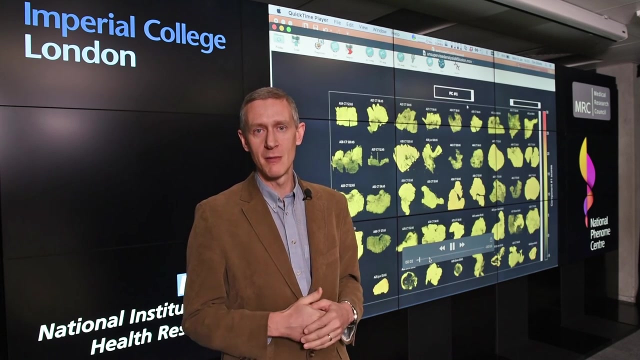 and computational and statistical techniques are being applied to solve biomedical problems such as finding the causes of cancer, for instance, or other diseases, And what we do here on the course is get students to study a programme composed of two long research projects, six months each, and a core programme of lectures and seminars and practical training. 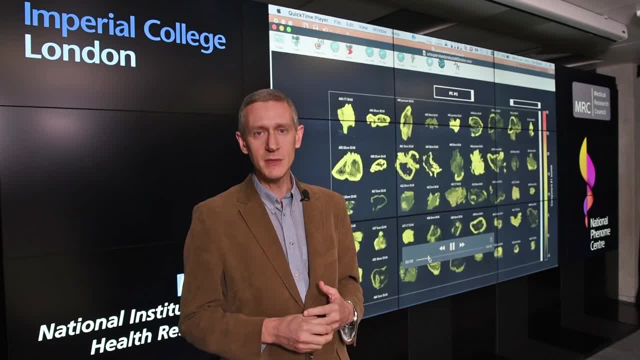 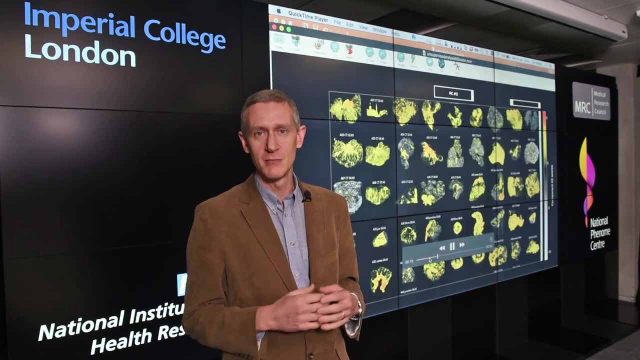 which will enable you to gain the right skills in both the computational work but also general research skills, to address these kinds of problems. going forward, Many of our students have left to go on to do more research in this area, such as a PhD, or they've gone to do 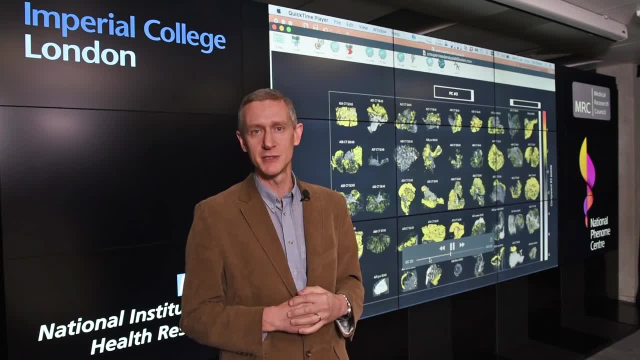 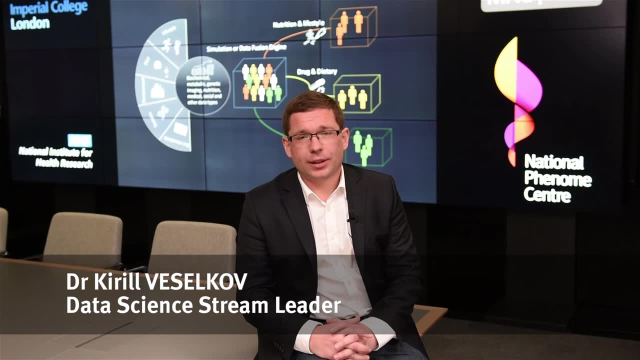 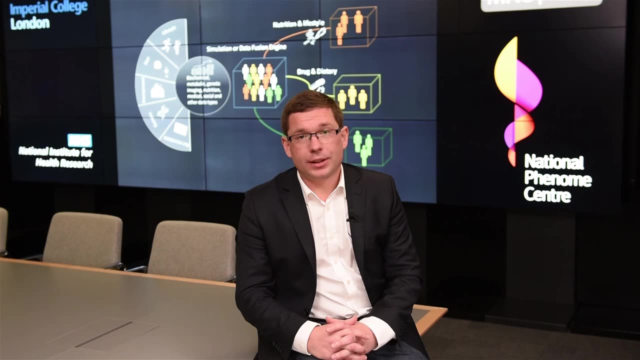 training in other areas or jobs in commerce and industry, such as finance, for instance. Digital technologies have enabled to capture human biology and activity in unprecedented details. In the not-too-distant future, various data from variable devices, medical records, genomics, metabolic technologies, as well as social media use would allow to build 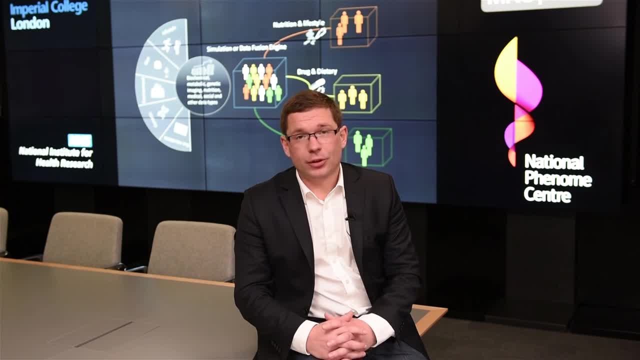 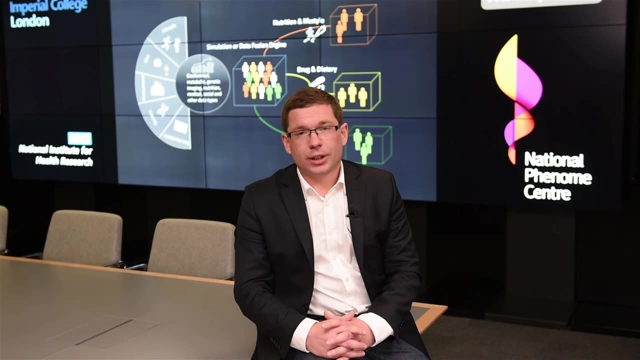 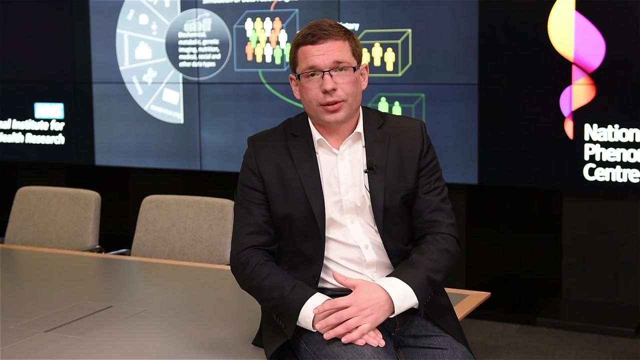 a comprehensive picture of a patient as an individual to provide more efficient, tailored healthcare. Data, in a way, is a commodity, and data science is a process of transforming unrefined data into meaningful, actionable insights to improve patient care. The data analysis course would allow you to build unique data analytical skill sets that are currently 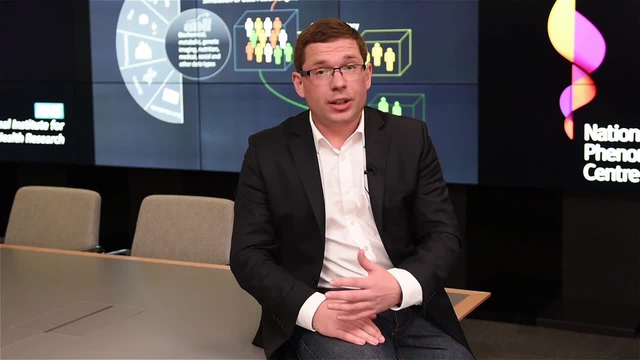 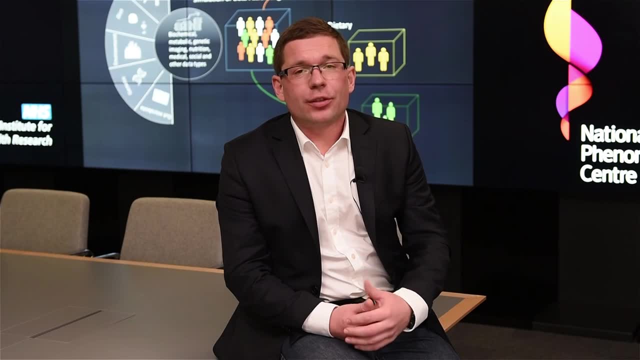 in ever-increasing demand in academia, in data-driven healthcare, in clinical research in healthcare, as well as various industries and businesses. The future lies in integration of digital, biological and physical worlds, and currently all major corporations, such as Facebook and Google, are investing a lot in digital healthcare.